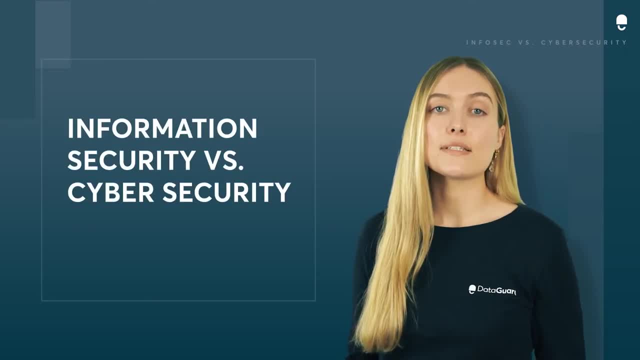 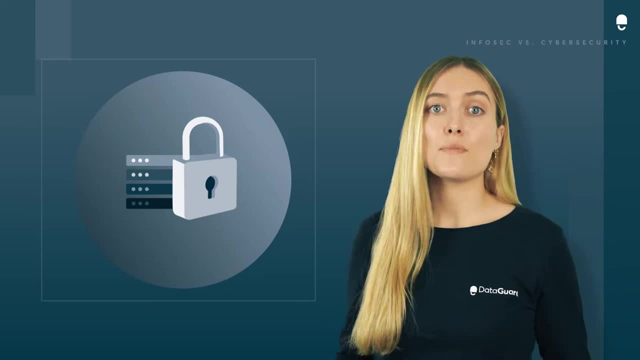 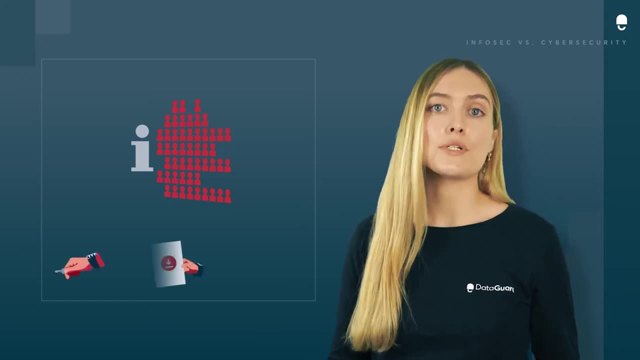 Information security and cyber security. what's the difference? The terms cyber security and information security are often used interchangeably, even among some of those in the security field, but they are not the same. When we think of data, we tend to think of computers and digital information. 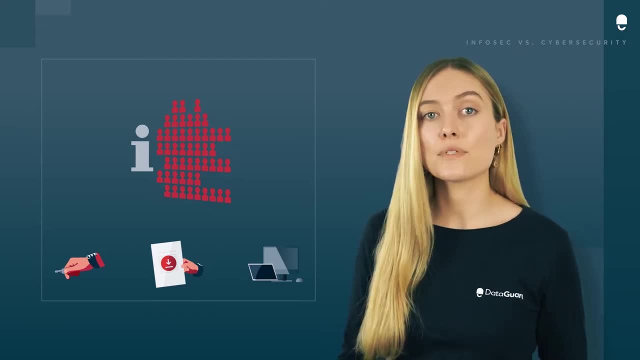 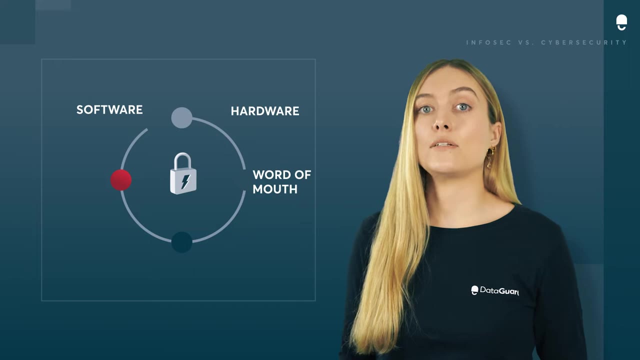 but meaningful, valuable data can be stored in many forms. Information security refers to protecting data, no matter what form- it's in digital or physical. Basically, information security is as much about protecting physical information or access controls like filing cabinets or physical access to building entrances. 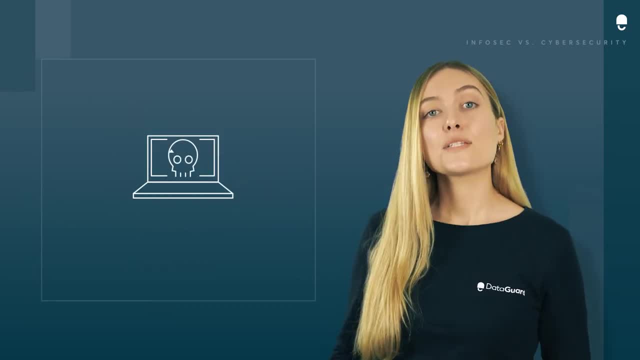 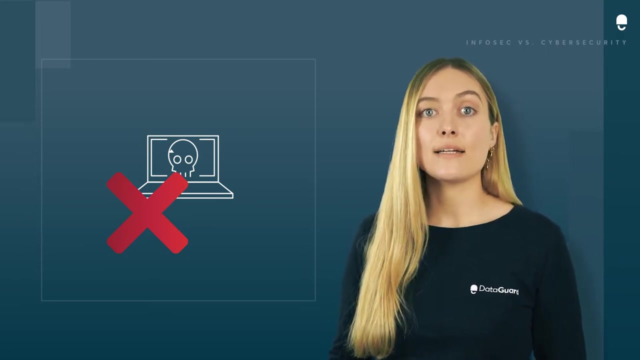 as it is about protecting databases. Cyber security is the steps taken to prevent cyber attacks from inside or outside your organization. It protects digital information that's stored on computers, devices, networks, servers and programs from hacking, a tax or an authorized access. So you can kind of view cybersecurity as a subset of information. 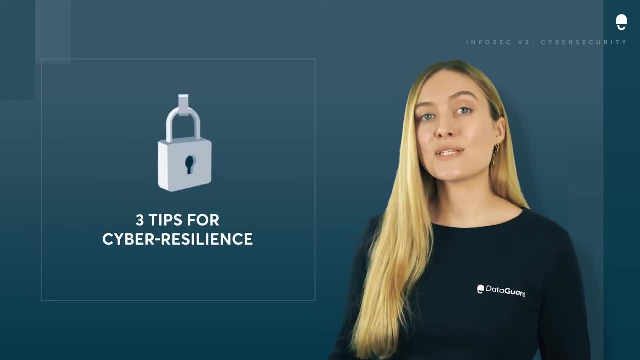 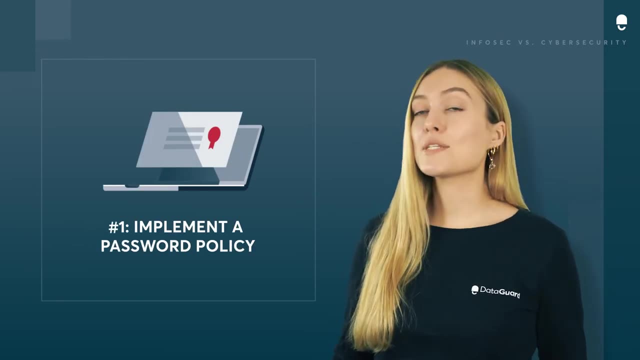 security. Here are three tips to make your business more cyber resilient today. Tip number one: implement a password policy and a password manager. Weak passwords are gold dust for hackers. Educating your team to use complex passwords or passphrases will make a massive difference to 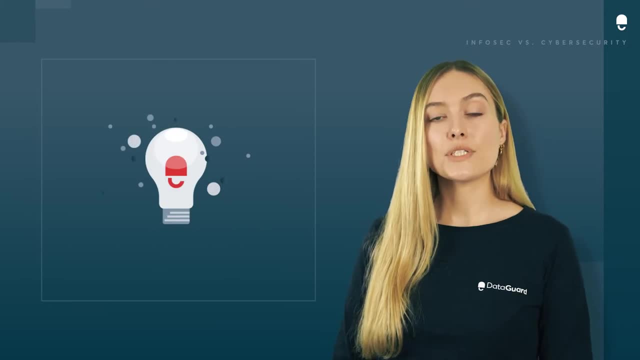 cyber resilience in the long term. To help your team out, you should also implement a password manager which allows your team members to store all of their passwords in a secure system, And it means they'll only have to remember one master password. Tip number two is regular pen. 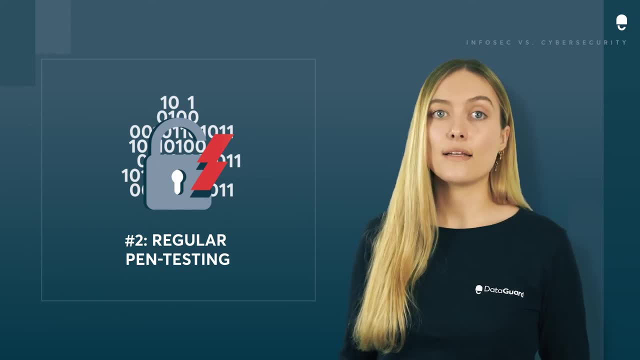 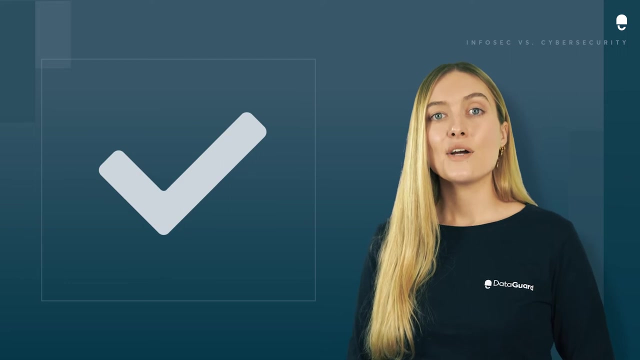 testing. A penetration test or ethical hacking is an authorized cyber attack on your systems which helps you to evaluate the security of those systems. This is a really brilliant way to identify weaknesses. Here at DataGuard, we've partnered with several pen testing providers and we highly recommend. 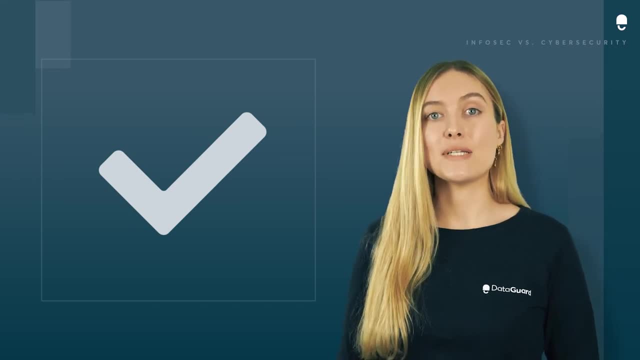 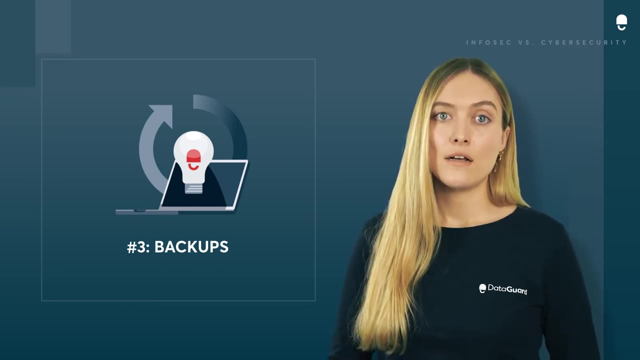 considering regular pen testing to boost the resilience of your business. Tip number three is backups. Backups are your business's lifeline if you ever do get hacked. Often hacks will result in your data being rendered inaccessible or corrupted. A good backup system will ensure that your business can continue to function even in the wake of a serious. 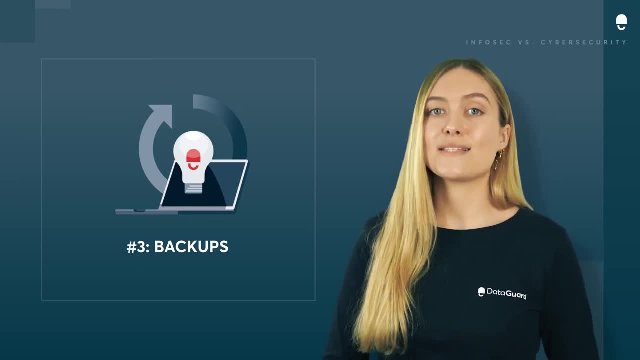 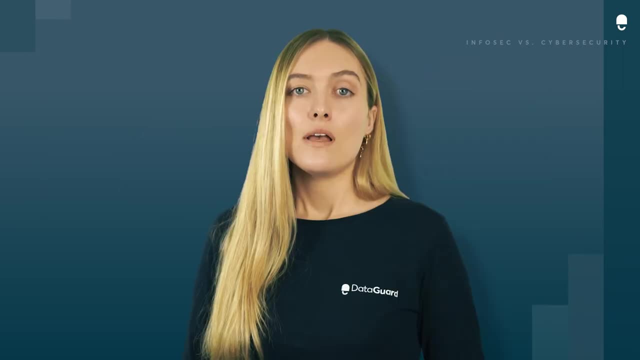 information security incident. In case I haven't stressed this enough, get your information backed up now. Your employees, customers and bottom line will thank you for it. If you're concerned about your company's information or cybersecurity status, then don't hesitate to reach out to us here at DataGuard. We would be happy to advise you. 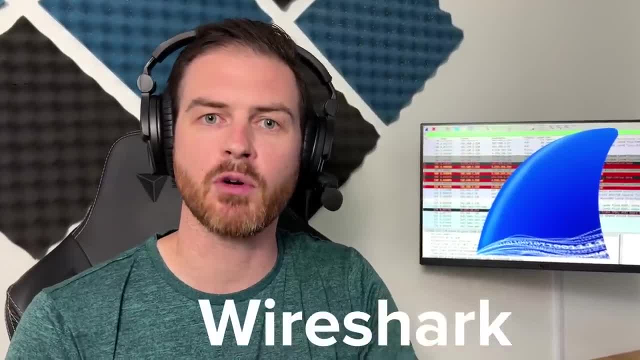 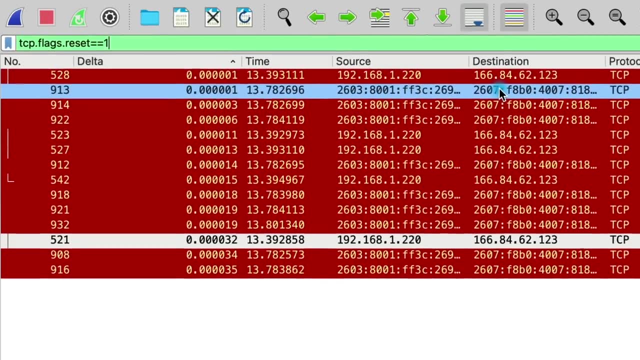 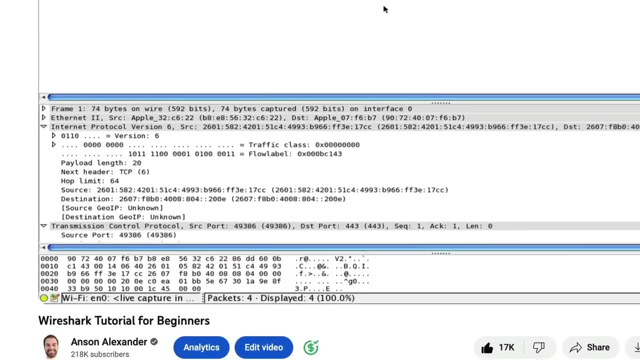 Wireshark is one of the most powerful network traffic analyzers for both Mac and Windows. I'm going to show you how to use it to view the traffic on your network, analyze packet data and identify any problematic or malicious activity. This video is an update to a Wireshark tutorial that I published over 8 years ago. 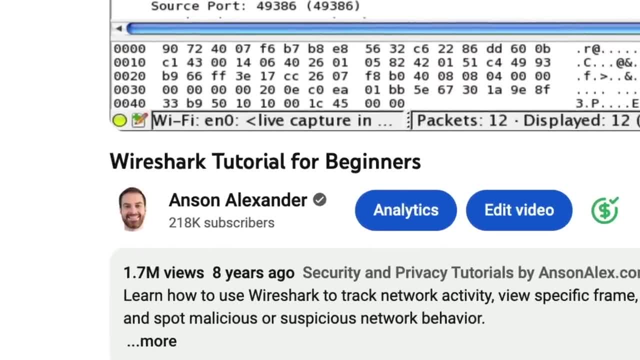 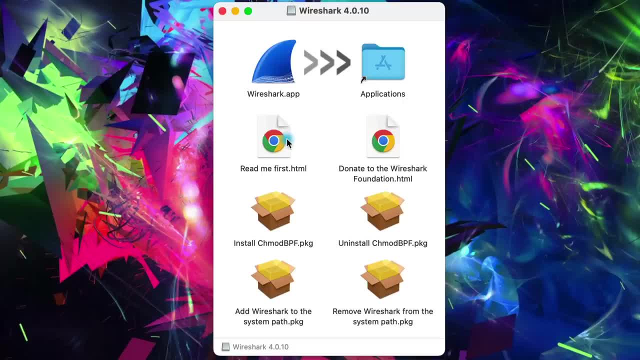 Since then, I've learned a lot more about Wireshark and cybersecurity in general, So let's get into it. Wireshark is free to download and use for both Mac and Windows. When you first install it, there's an additional package that you also have to install. 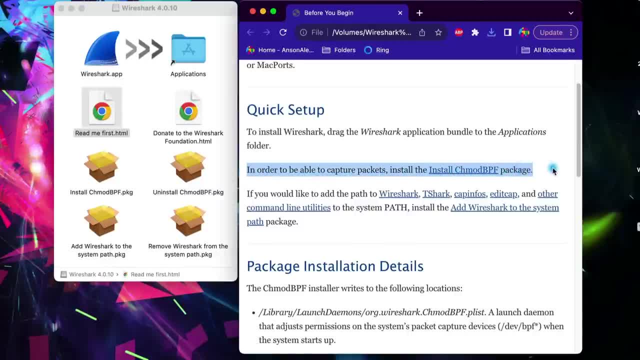 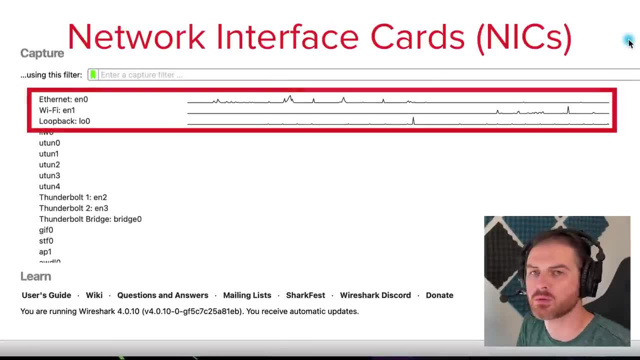 at least on Mac. So just make sure to read the README files that you see when you first download it. Now, once it's installed and open, you can immediately see in the capture section which network interface cards are picking up traffic. You obviously have to be connected. 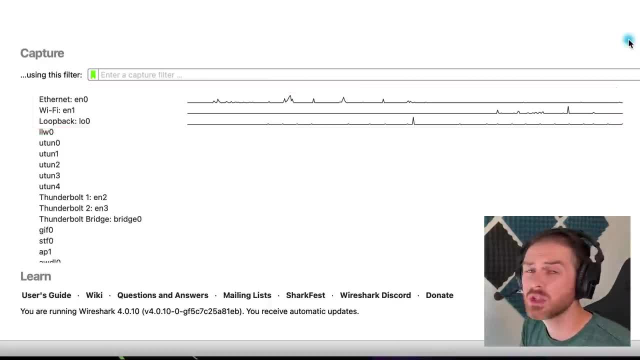 to the networks that you want to look at with the device, the computer that you're using. Generally speaking, you're going to want to look at your Ethernet or your Wi-Fi, Depending on your hardware setup. it can be difficult to sniff the packets on a Wi-Fi. 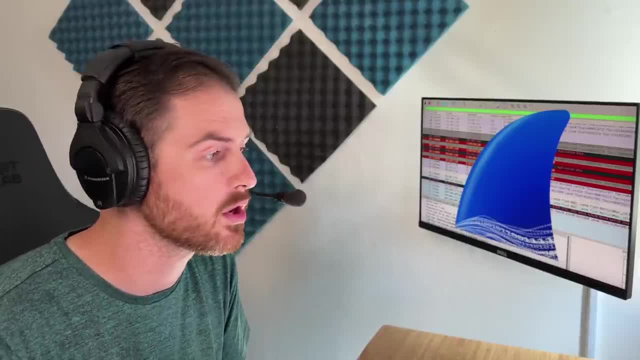 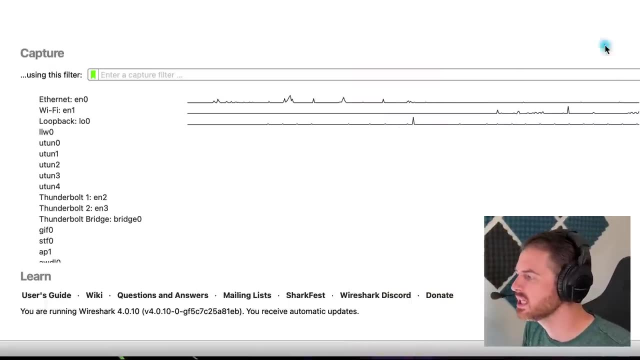 network Mac users should be totally fine. They have been for a long time with Wireshark able to do that. There has been some issues with Windows in the past, So to get started and just to jump right in and make sure we're getting good data. 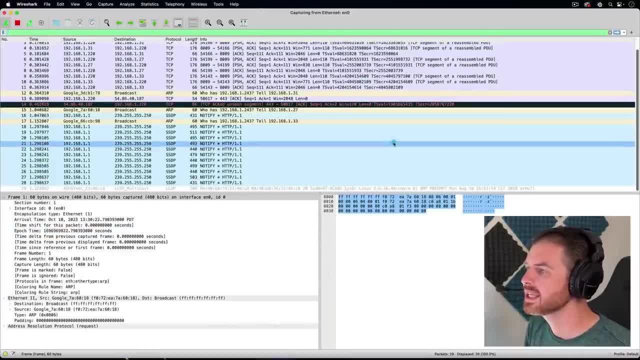 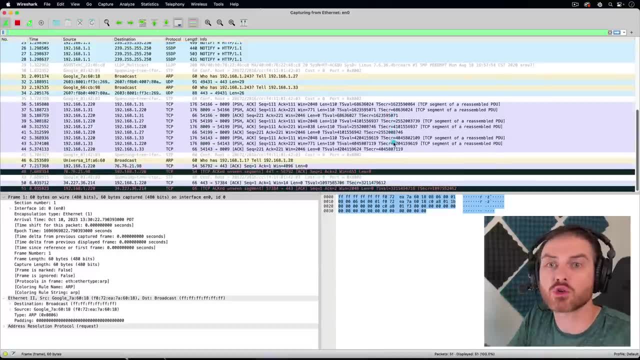 let's just double-click on Ethernet to take a look. When we double-click, immediately Wireshark starts capturing packets And we can let it go and capture packets for as long as we'd like. So if you're troubleshooting a particular website or something like that, you'll want. 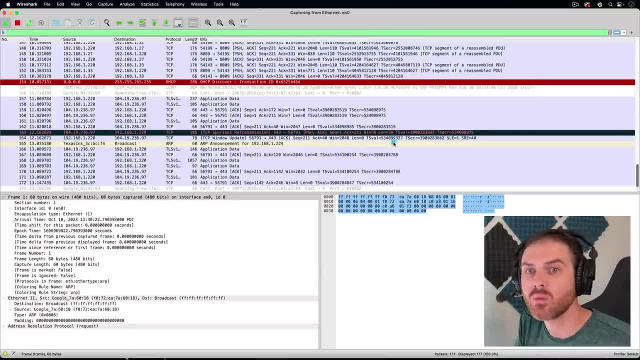 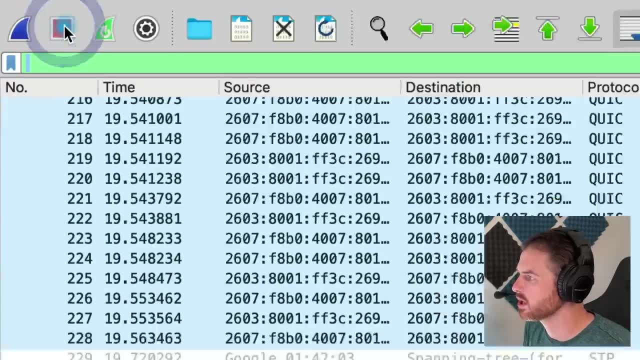 to try and access that website now while it's capturing, And then, once you think you have enough data, once enough time has gone by, you can go ahead and you can click on the red stop button up here at the top left. So now we have some information to work with.